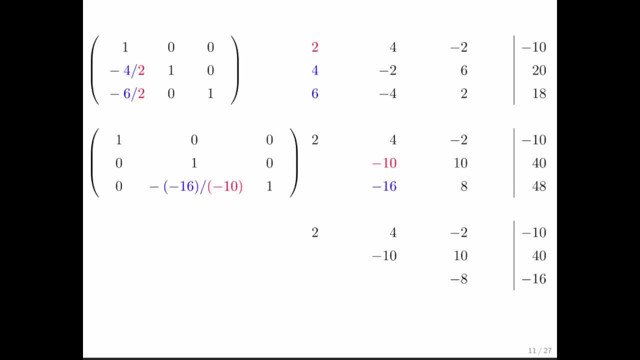 Or an upper triangular appended system, Or whatever you want to call it. Now we could simply forget about the right-hand side Because, remember, when you do a matrix, matrix, multiply, You can think of that as multiplying times, the columns separately, And therefore what happens is not going to be impacted at all. 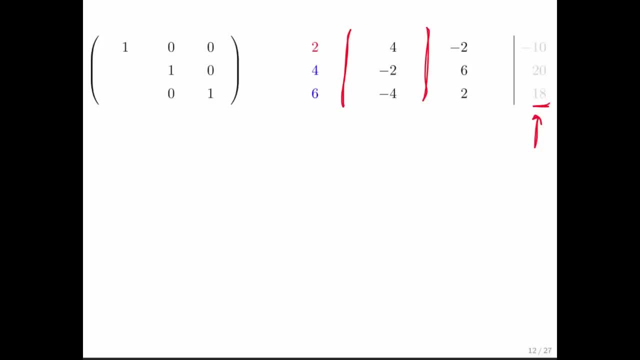 By how the Gauss transform is applied to the right-hand side. So what we can do, then, is compute our entries in our Gauss transform, Apply the Gauss transform to only the part of the appended system to the left of the vertical line, In other words to the matrix. 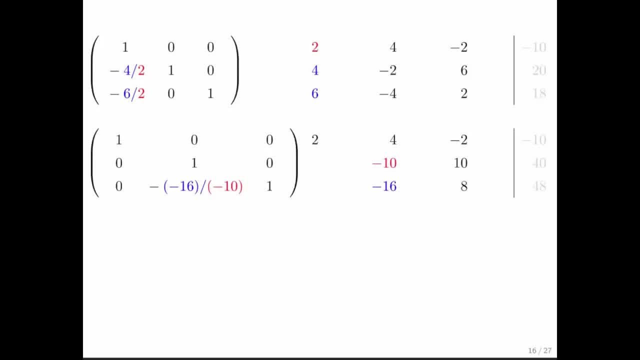 And then we can do that again. We can compute the entries in the Gauss transform, Apply it And we're left with an upper triangular matrix. Now, here we didn't actually write the zeros, But you can imagine where the zeros are. Then, if we stored the Gauss transforms, 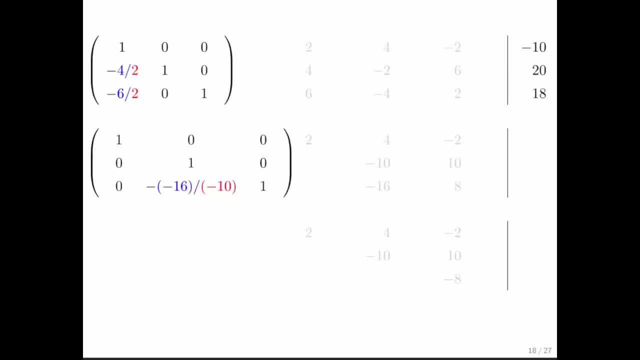 Then we could, a posteriori, after the fact, come back And apply those to the right-hand sides, To the right-hand side, To have the same net effect as if we had done so when we were working with the matrix Earlier And when we were actually computing those Gauss transforms. 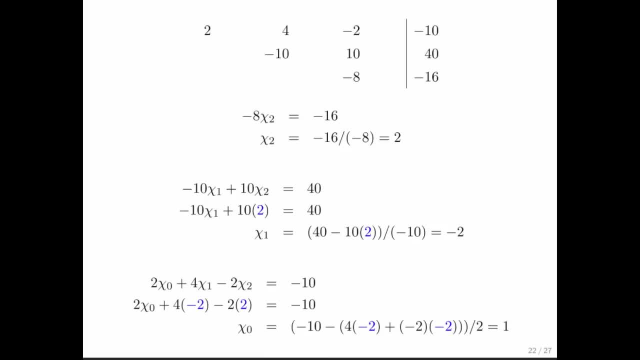 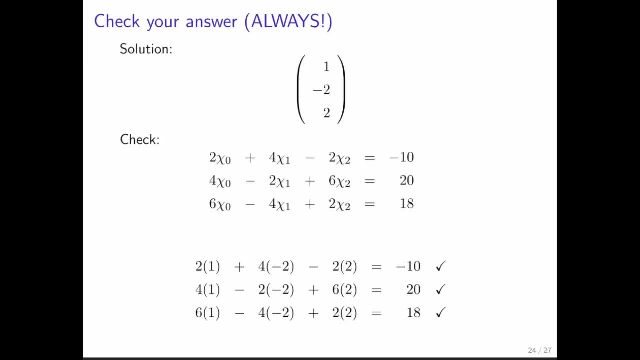 Then we can go on and do our back substitution And solve the upper triangular system. As always, check your answer. So what we have now is a systematic way for transforming the matrix to an upper triangular matrix. If we then store the Gauss transforms, 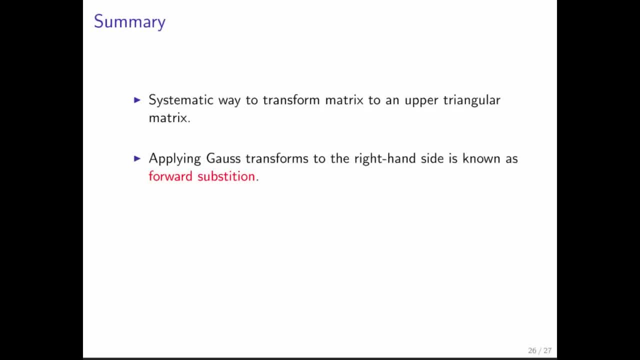 We can apply those to the right-hand side After the fact. This is known as forward substitution, Which I misspelled here- And notice that if then later on with the same matrix a new right-hand side comes along, You don't have to actually go and perform Gaussian elimination. 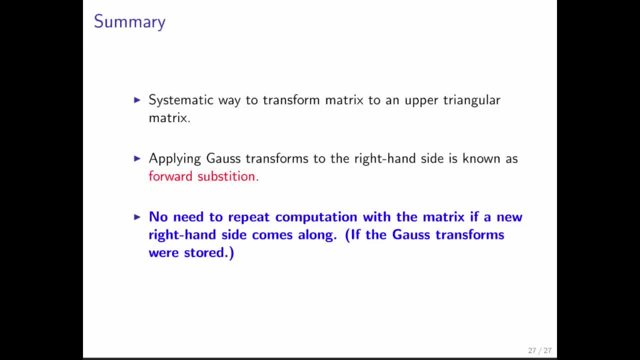 This reduction to an upper triangular matrix. With that matrix All you need to do is store the Gauss transforms So that you can do forward substitution with the new right-hand side.